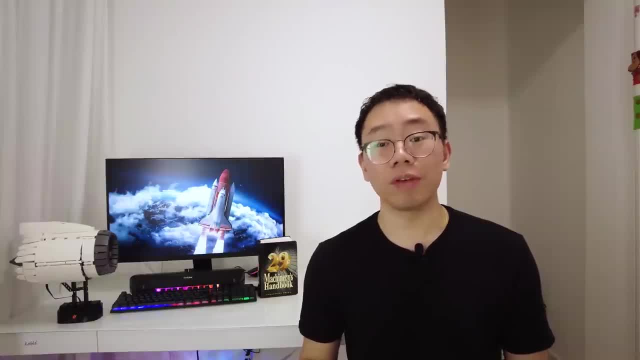 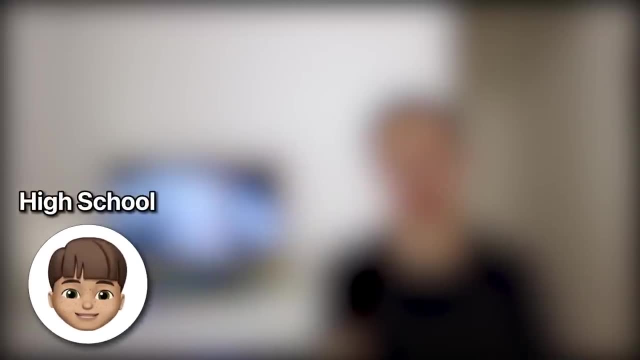 interests and values. Now, if you're watching this video, you probably fall into one of the following categories: You're currently a high schooler deciding between the hundreds of majors out there. You're a university student thinking about switching over from, perhaps, software. 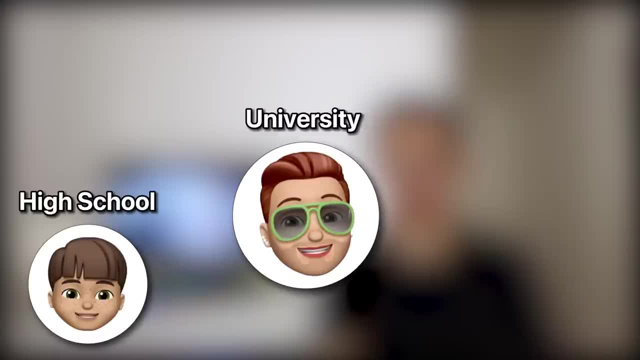 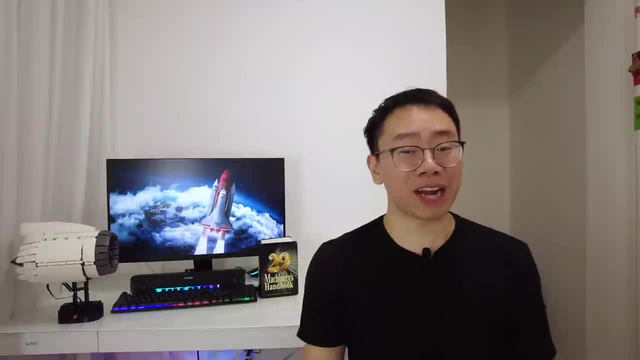 electrical or chemical engineering or a non-engineering major to mechanical engineering, Or you're currently a working professional and planning to attend grad school for mechanical engineering. Whichever category you fall in, it doesn't matter, because by the end of this video, 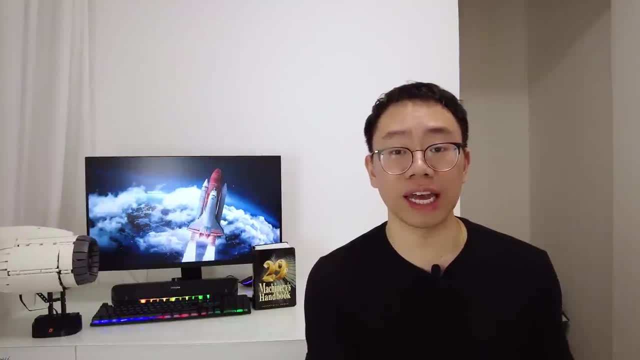 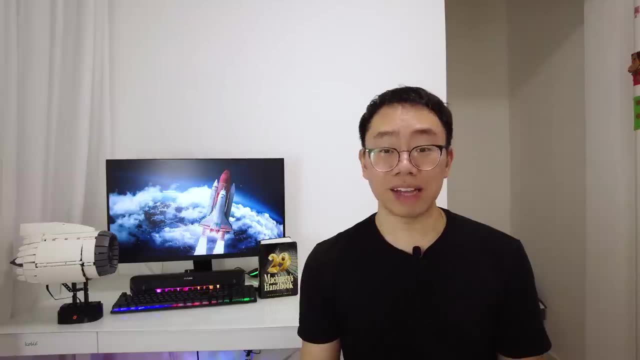 you'll know exactly whether you should or shouldn't get into mechanical engineering. The first question that you should ask yourself is: do you like math and physics? You don't have to have a burning passion for these, but you have to be at least willing to sit down, learn the 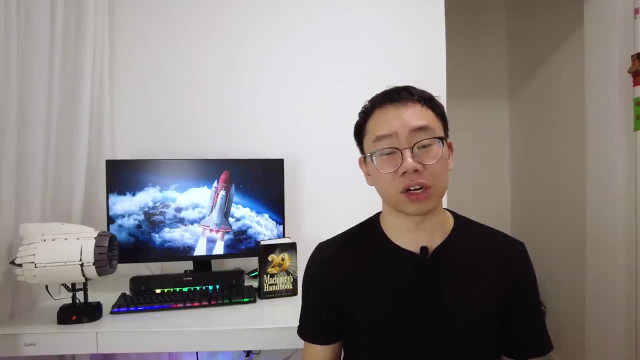 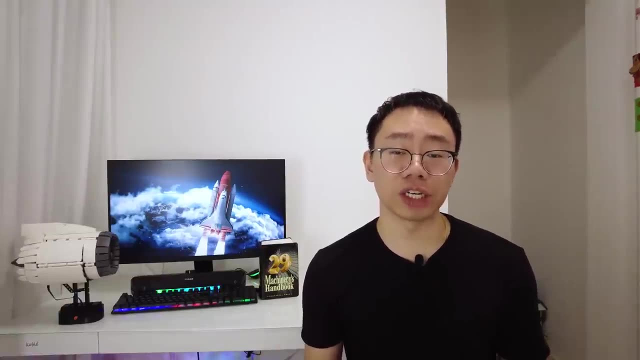 material and practice. What I've noticed is, the best engineers are the people who are the best, people who truly enjoy math and physics in school. After all, math and physics form the foundation of mechanical engineering principles. You have to take a plethora of math classes like 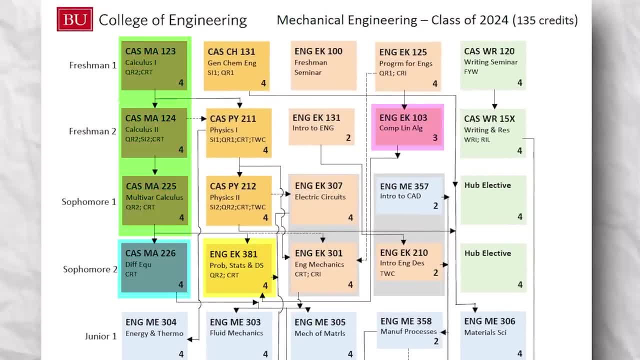 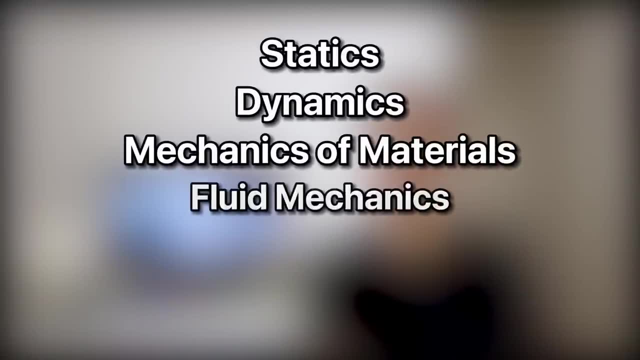 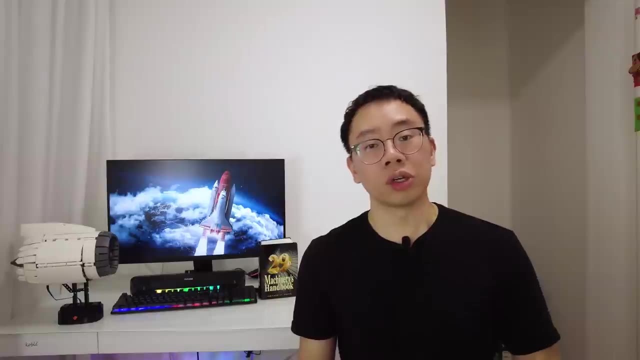 calculus, differential equations, statistics and linear algebra. in undergrad, Many of the core mechanical engineering courses like statics, dynamics, mechanics of materials, fluid mechanics, thermodynamics and heat transfer leverage physics principles and concepts to solve engineering problems. So if you absolutely hate math and physics, you should definitely go to 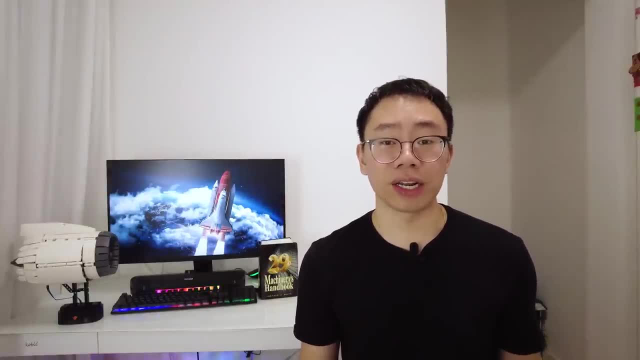 math and physics. Definitely avoid mechanical engineering- and engineering in general for that matter- at all costs. It's totally okay if you're bad at math and physics, so long as you find different ways to improve. The second question you should ask yourself is: are you interested? 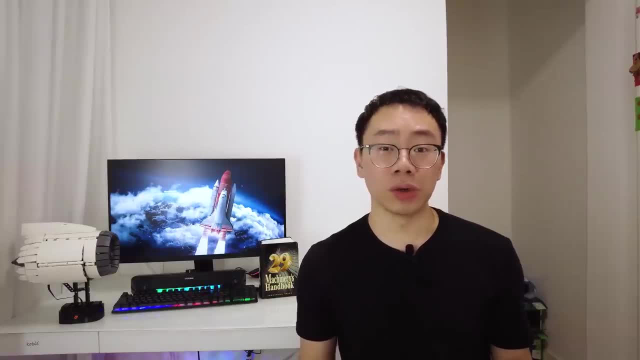 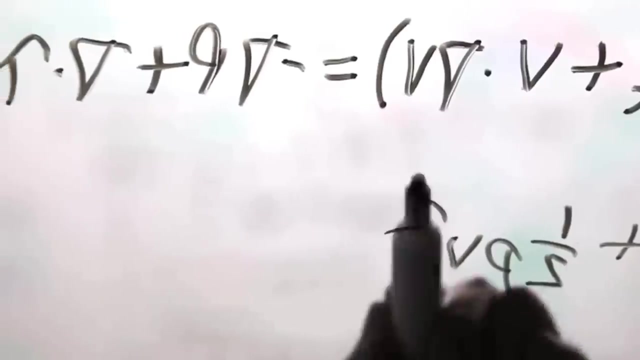 in creative thinking, If you like, being told what to do and borrowing ideas from others without doing the thinking yourself. mechanical engineering will be challenging and is likely not for you. Most people think hands on and technical skills or mathematical prowess when they think engineer. However, creativity is. 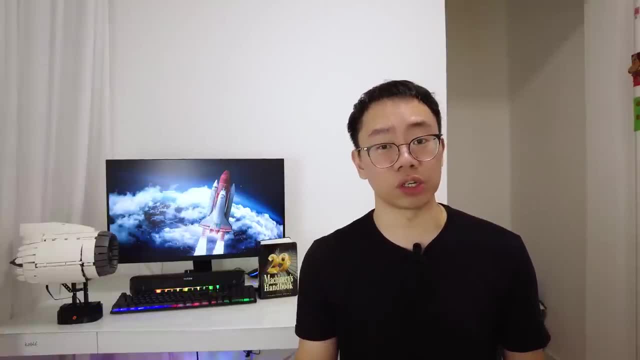 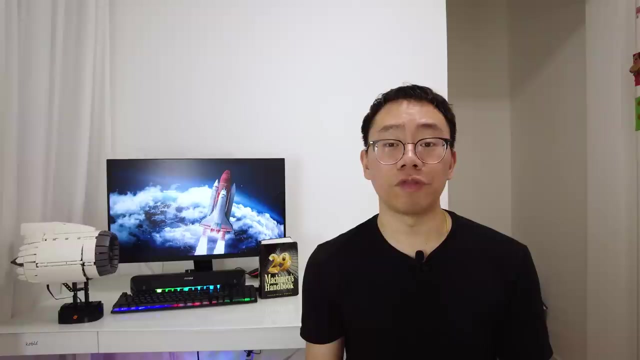 just as important, especially for mechanical engineers. Creativity might not seem as important in university, but once you get into industry it will be a huge game changer. A huge part of a mechanical engineer's job is to design products such as an iPhone, Tesla or jet engine following. 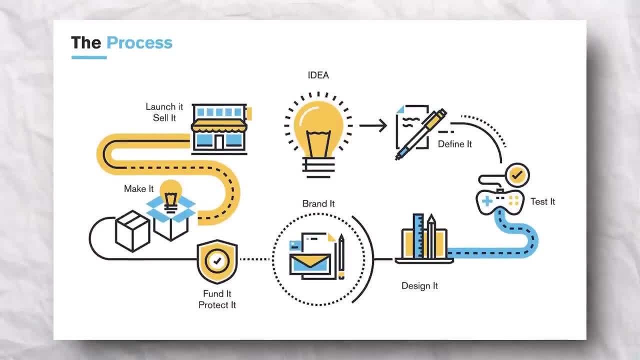 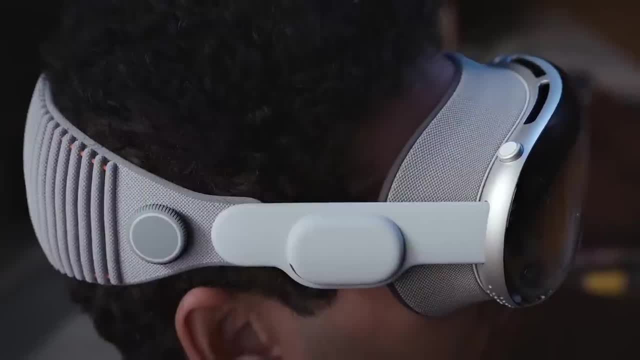 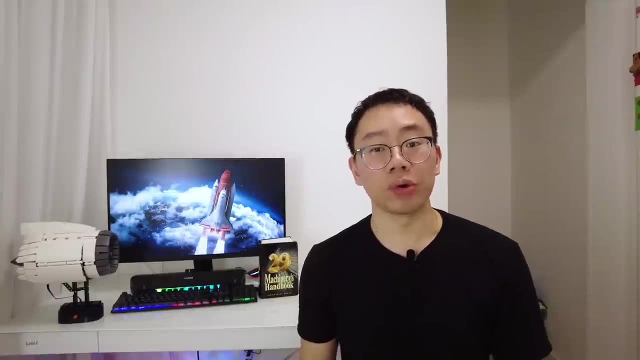 the product development process. The first stage of this process is the ideation phase, where you come up with a bunch of design ideas and evaluate them using a pew chart. Creative thinking helps in generating innovative designs that are functional and ergonomic. Once you have a concept, you will 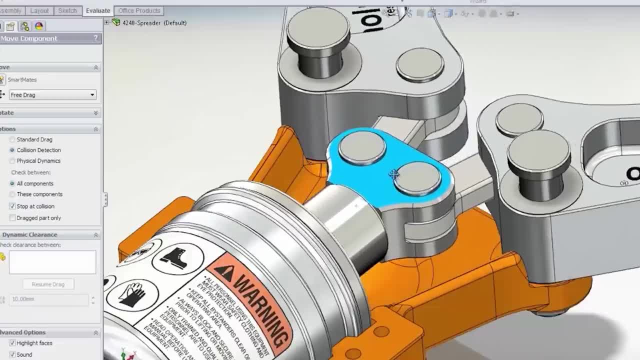 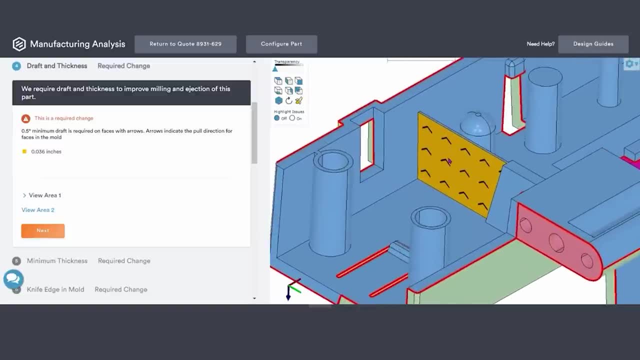 need creativity to engage in the high level and detailed design of components and assemblies using CAD, including mechanical features like holes, screw bosses and ribs, as well as the overall system design. Along the way, you'll encounter all kinds of challenges that require you to think. 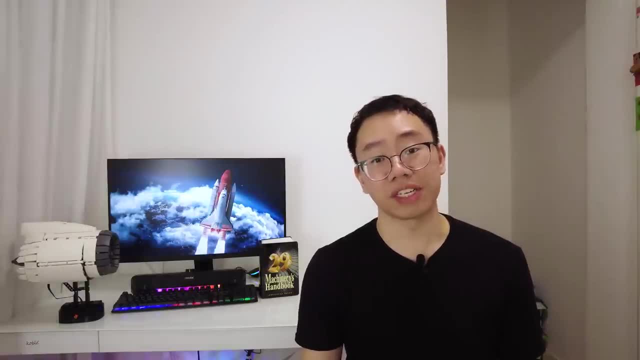 outside the box. If you're a mechanical engineer, you'll need to think outside the box. If you're a designer, you'll need to think outside the box and find novel solutions to address them. For example, if you found out that the parts you designed don't fit together, you need to be. 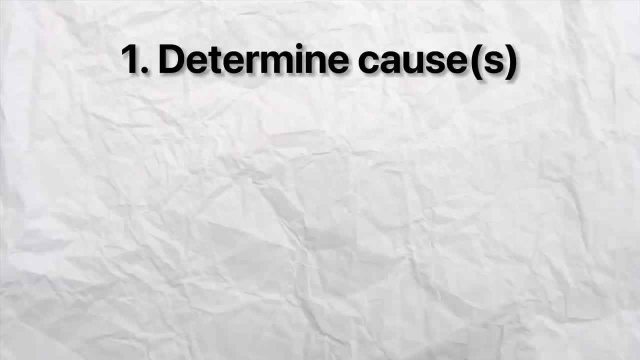 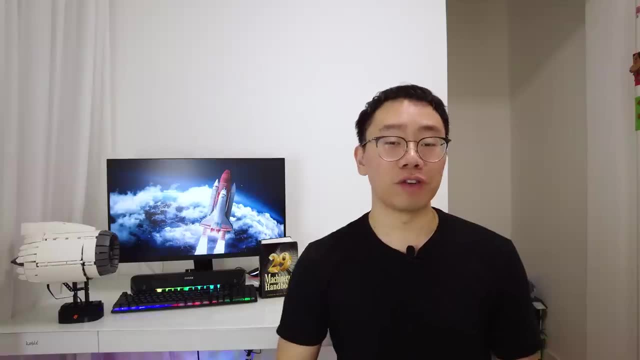 creative and find an effective method for determining the cause- whether it's related to tolerances, faulty design or a manufacturing defect- and proposing a corrective action. So if you're opposed to creative thinking, you should not get into mechanical engineering. However, 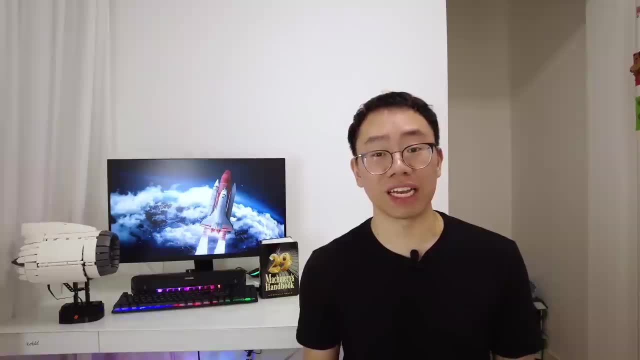 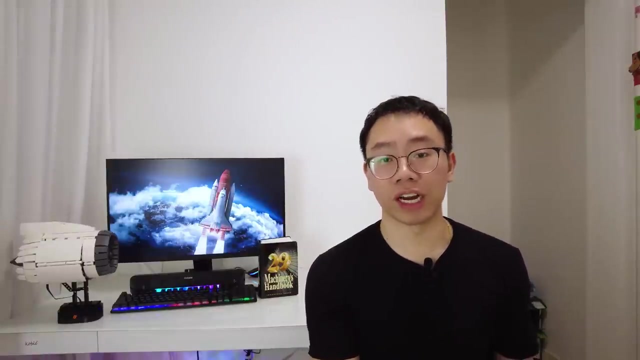 if you're open to the idea of engaging in creative thinking on a regular basis as part of your job, you can still become a mechanical engineer. Luckily, creativity is a skill that can be developed and learned over time. The science shows that a lot of things promote creativity. Some things that I like: 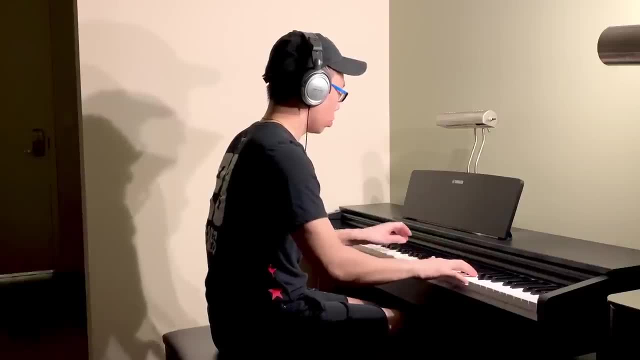 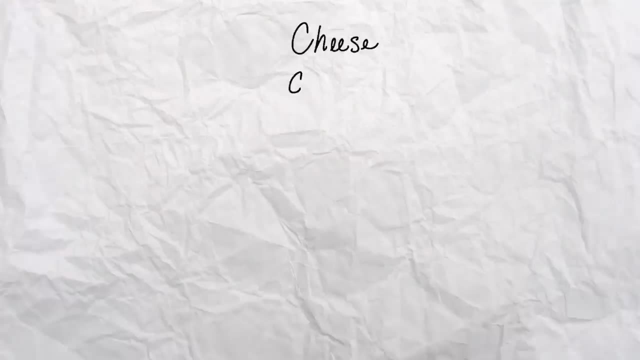 to do that. help with creativity include playing an instrument, reading books, working out in the gym or even playing games like Drawful Pictionary or that game where you write down as many words that you can think of that start with a specific letter or phrase If you're open to creative thinking. 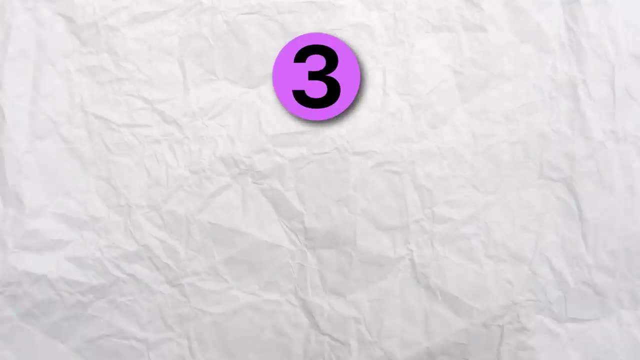 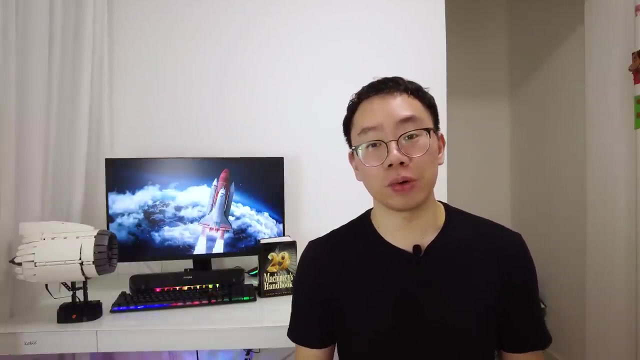 you can still get into creative thinking and you can do the same things that you're used to. 3. Do you like hands-on work? Mechanical engineers are portrayed in movies as people who have a knack for designing and building their own gadgets from scratch- like Tony Stark, Of course. 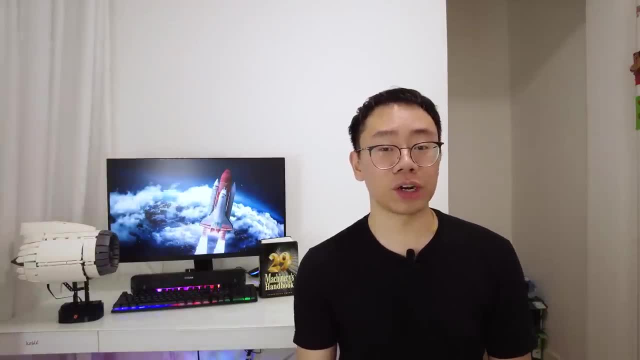 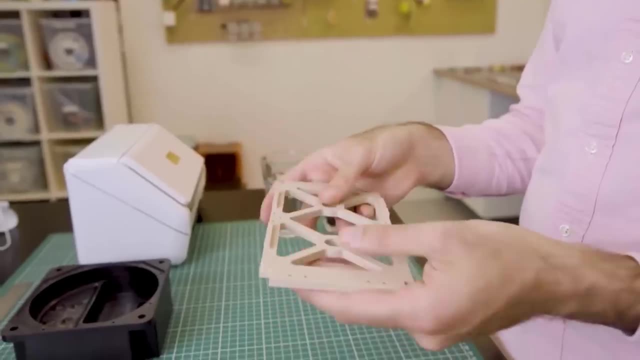 things in movies are exaggerated, but mechanical engineers, in addition to working in the office, almost always do in fact work in a hands-on environment like a test lab, machine shop or manufacturing plant to build, and they can be really creative. The question is: 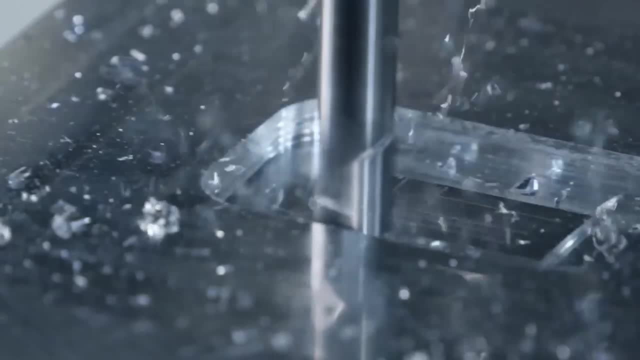 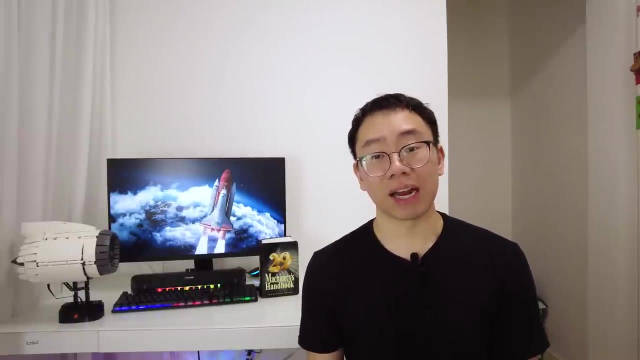 and test prototypes and products leveraging various machines and tools. keep in mind that some jobs will definitely be more hands-on than others. for my first full-time mechanical engineering job in boston, massachusetts, i spent about 50 of my time in the office and the other 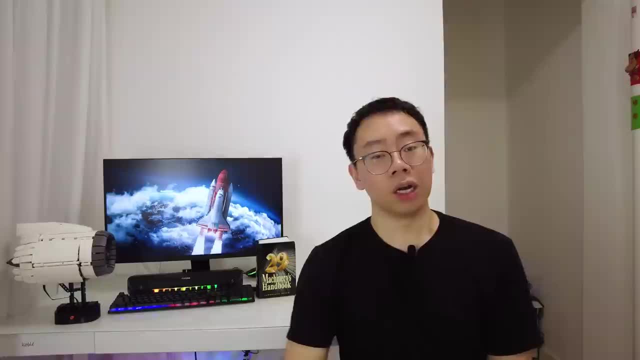 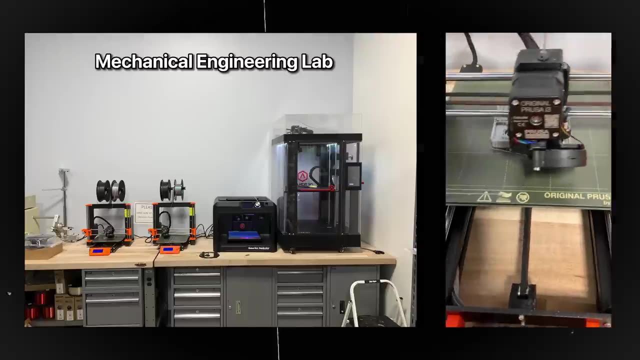 half either on the shop floor or the mechanical engineering lab. aside from all the typical mechanical engineering work we did on a computer in the office, we used 3d printers to print prototypes, proof of concepts and test fixtures, as well as build automated testers. we also had our 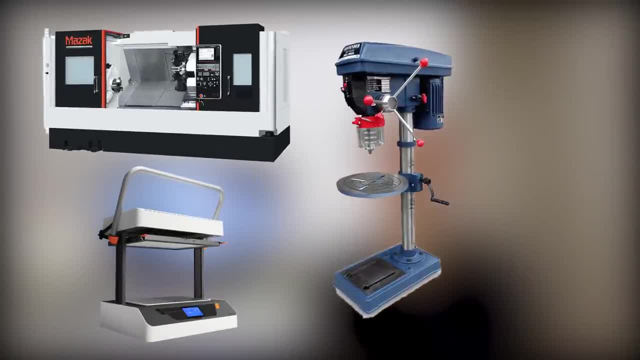 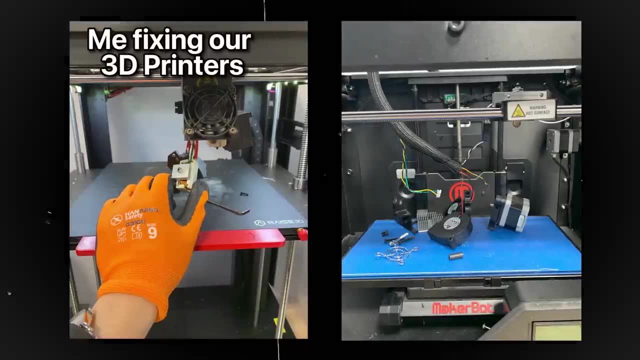 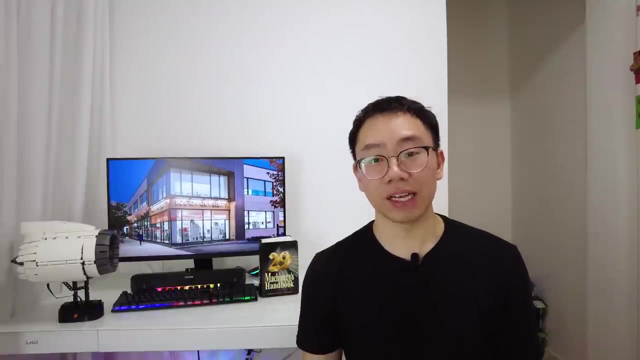 own cnc machine, drill press, vacuum forming machine and bandsaw that we used to make our own parts. when these machines broke down, we were responsible for getting them back up and running again because our company was too stingy to hire technicians. then, at my second job in silicon valley, there was 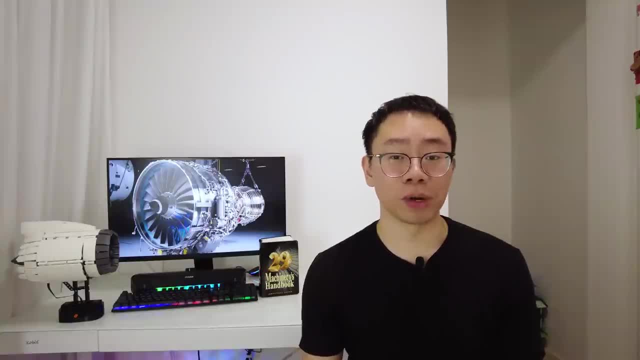 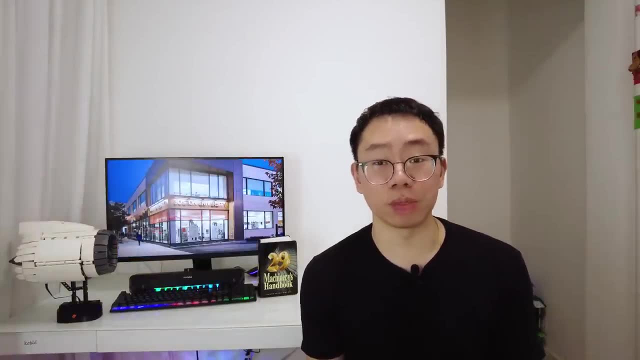 literally zero hands-on work and we just sat in front of a computer all day, which is uncommon from what i've seen so far in the past few years. i've been working on a computer for a long time- mechanical engineering jobs- so if you dislike hands-on learning and working with tangible 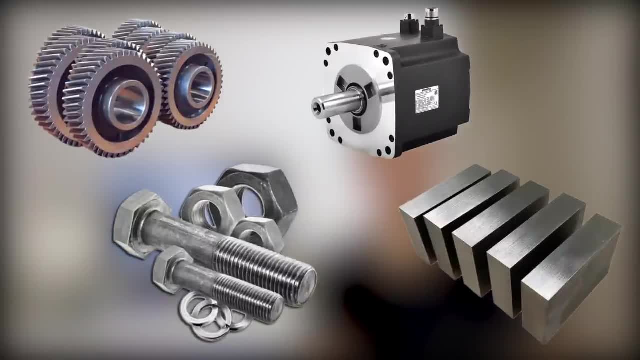 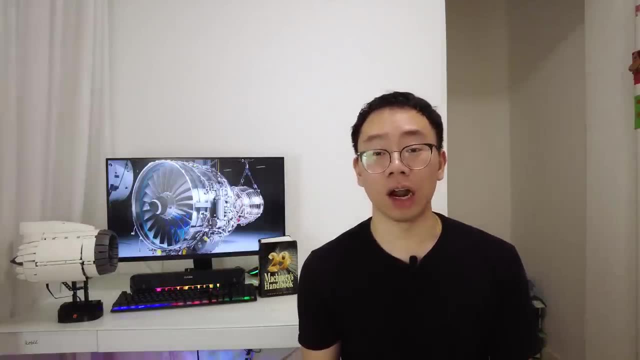 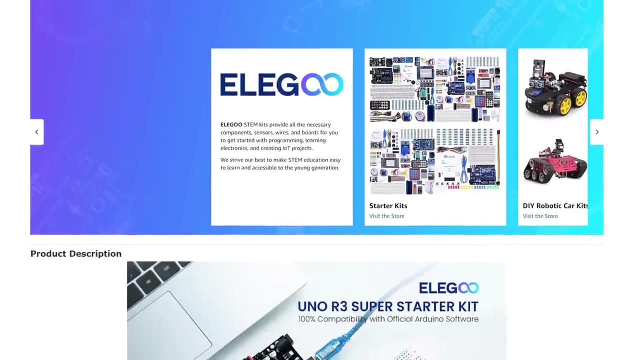 things like gears, fasteners, motors and raw material, then mechanical engineering is definitely not a good option for you. there are many ways to improve your hands-on ability if you're currently in high school or university. the elego or arduino kit on amazon is great for learning about circuits, motors and coding, which are all important. 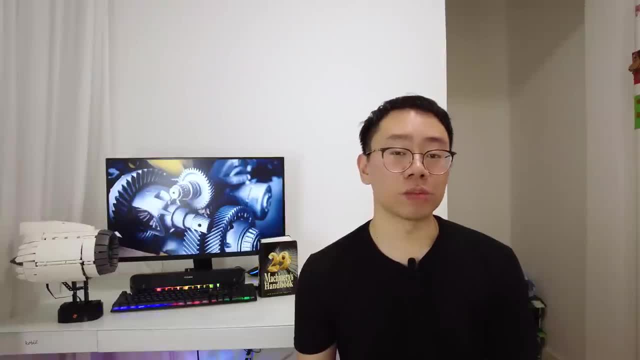 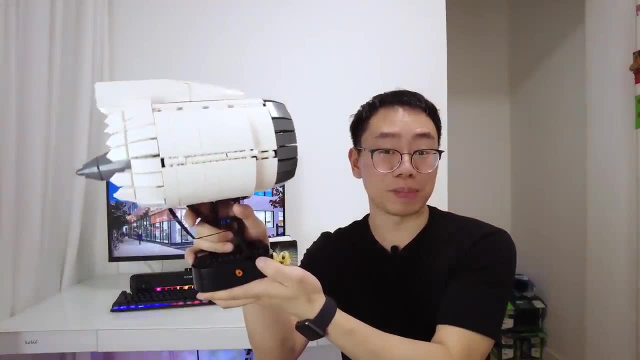 things to know as a mechanical engineer. i'll drop a link in the description below for any of you who are interested. also, if you're a gearhead and into engines and building things, like me, then i highly recommend checking out medieval bricks. they offer a wide selection. 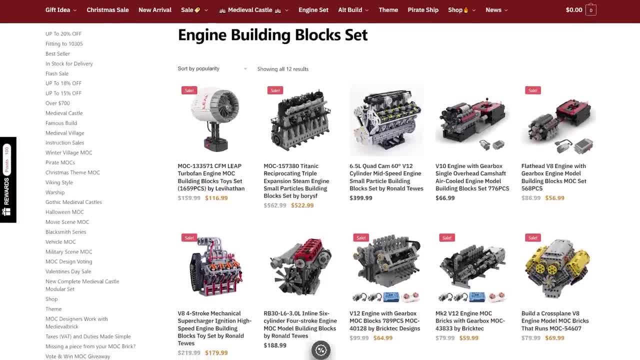 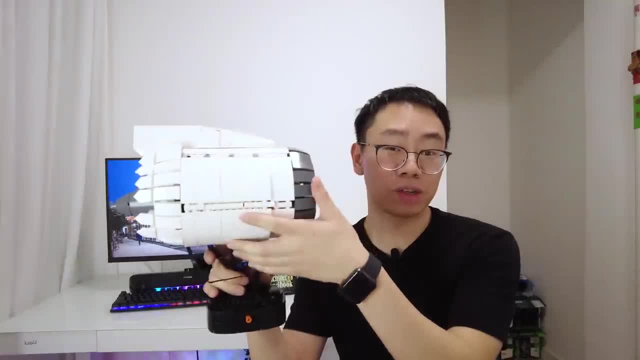 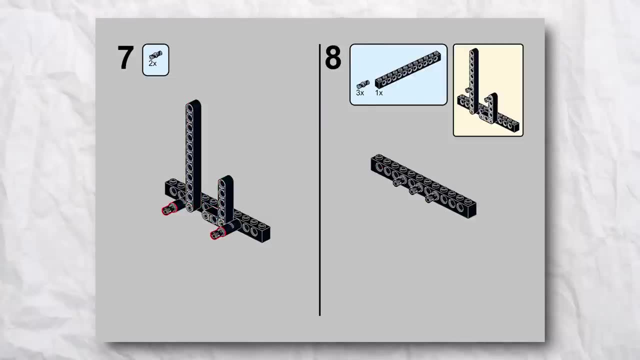 of very realistic engine building block sets from a quad cam v12 cylinder engine to a titanic triple expansion steam engine. i picked up this 1600 piece turbofan jet engine set for christmas and it took me about a week to assemble. all of their kits include a step-by-step 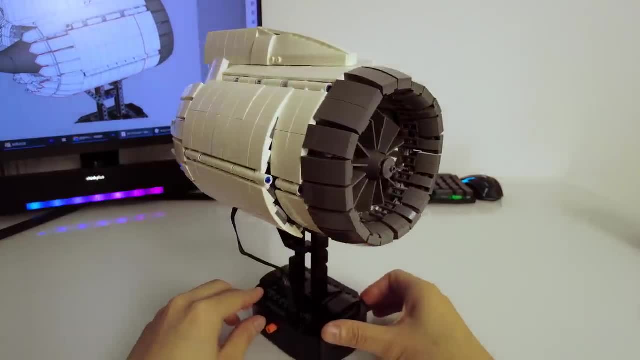 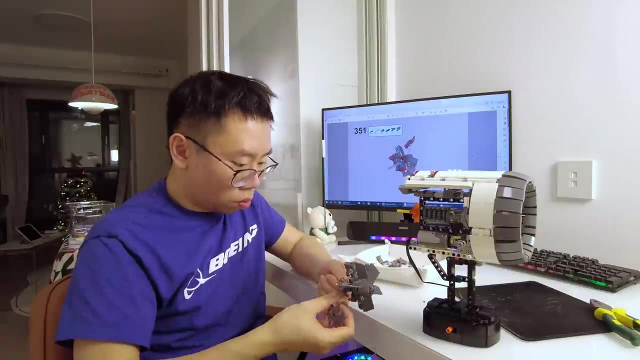 assembly manual like this. by the way, this video isn't sponsored. i just wanted to share this with any of you looking to get your hands dirty and have some fun. the kit i got was one of their more challenging ones to assemble, but they offer kits with around 600 to 700 pieces. for those of you who 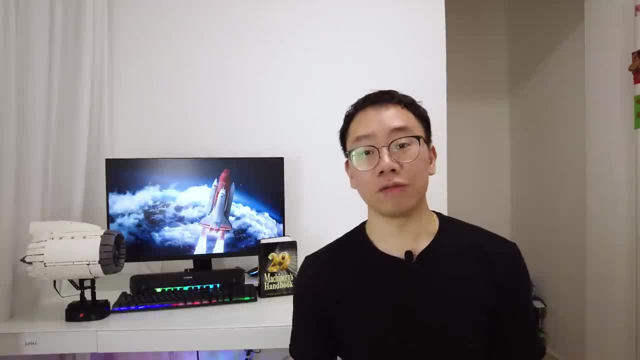 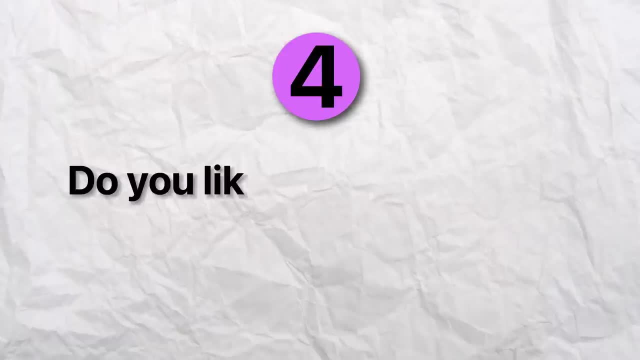 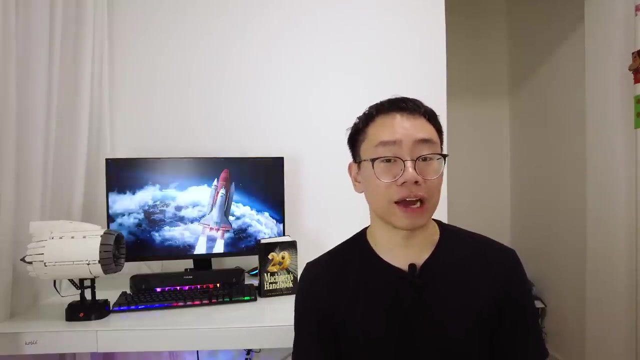 are less patient and just want to get something built. so for any of you who are interested, definitely check out my link in the description below question 4. you need to ask yourself is: do you enjoy the process of solving complex problems? do you find satisfaction in figuring out solutions to intricate, complex engineering challenges? 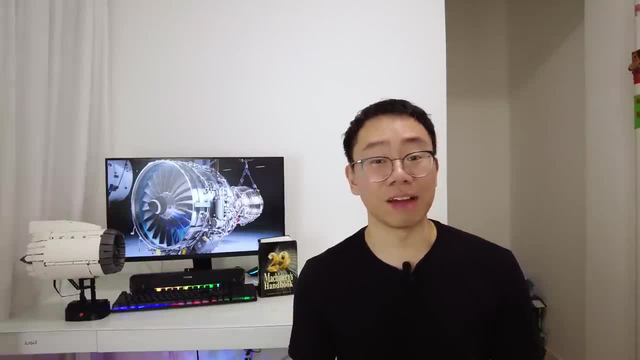 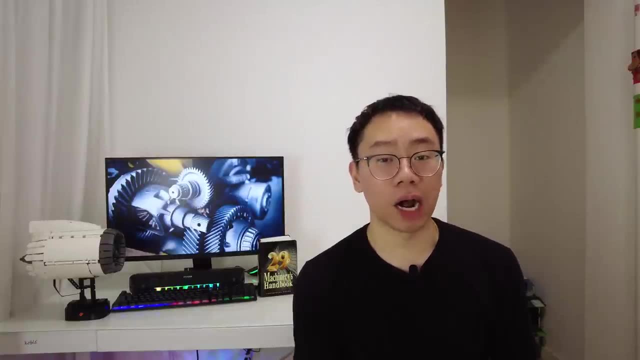 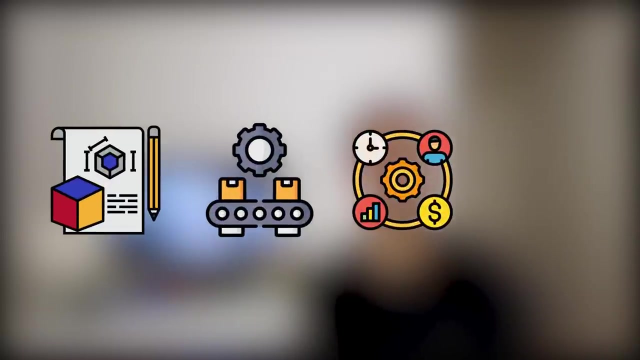 the job of any engineer boils down to solving different types of problems, whether related to products or processes. as a mechanical engineer, you'll come across problems that you would never imagine or deal with in school, related to product design, manufacturing, project management, budgeting and dealing with it in university. you'll also be problem solving a lot, whether it's on 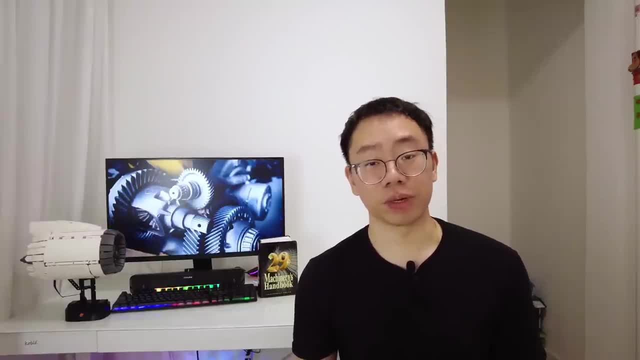 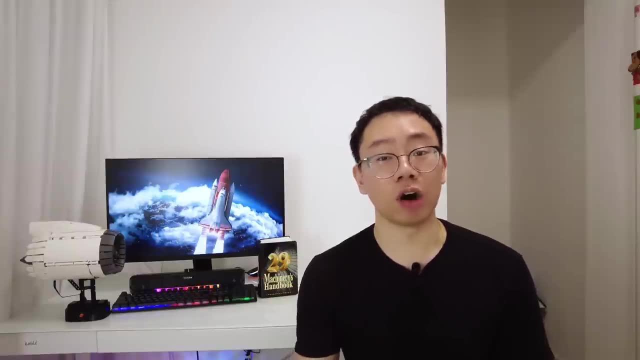 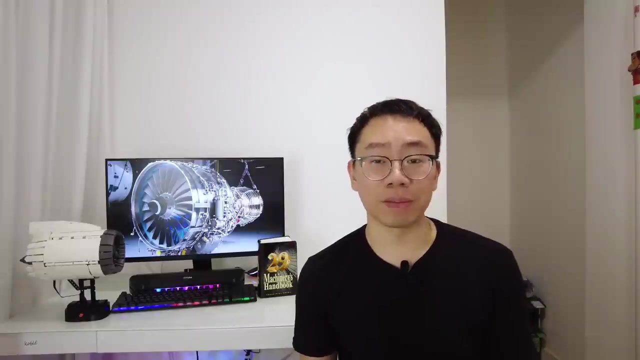 homeworks, design projects or research. the biggest difference between problem solving in school and industry is that real world problems are much more ambiguous and multi-faceted, involving technical aspects as well as economic, social and environmental factors. there will also be time, budget and resource constraints. problems in school are generally well defined, with known parameters. 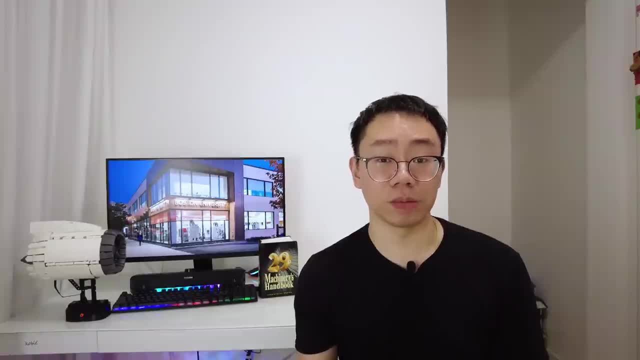 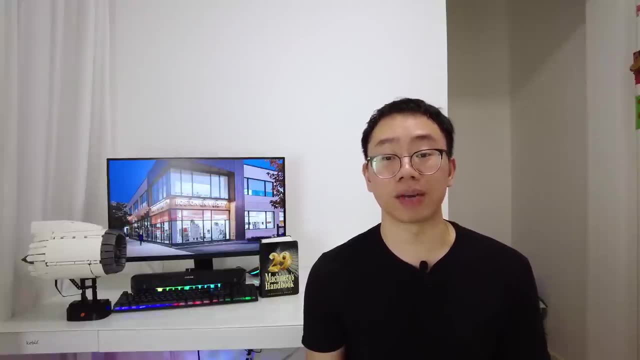 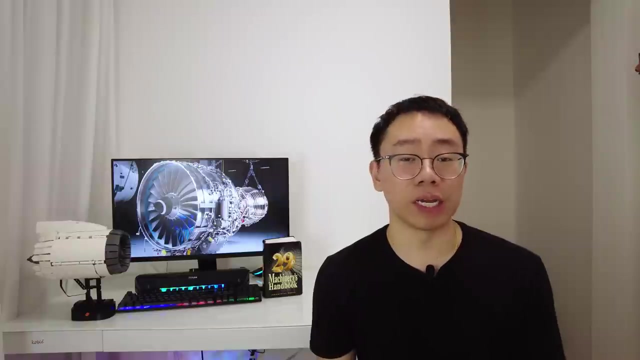 and very few constraints aimed at teaching specific principles or concepts. so it's without shame. you'll be solving problems on a regular basis if you do get into mechanical engineering. next, ask yourself: what are your career goals? if your primary goal is rapid career entry without getting a degree after high school, then mechanical engineering is not a good choice, unlike some. software engineering roles that don't require a degree. all mechanical engineering roles require you to hold a bachelor's degree or higher. however, if you're considering mechanical engineering, you're probably already planning on going to university. you're probably already planning on going to university now if you're someone who plans to make six figures as a mechanical engineer straight out of. 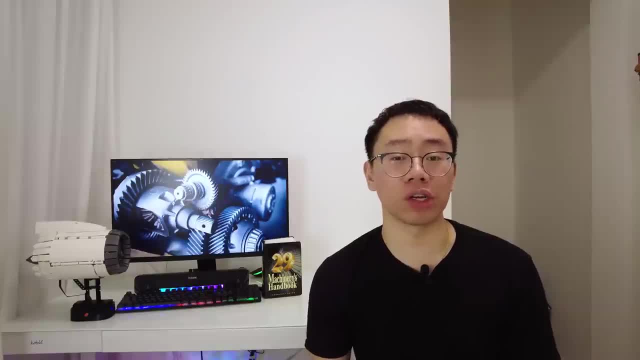 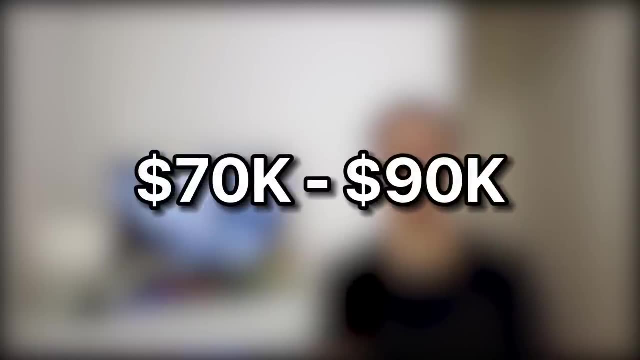 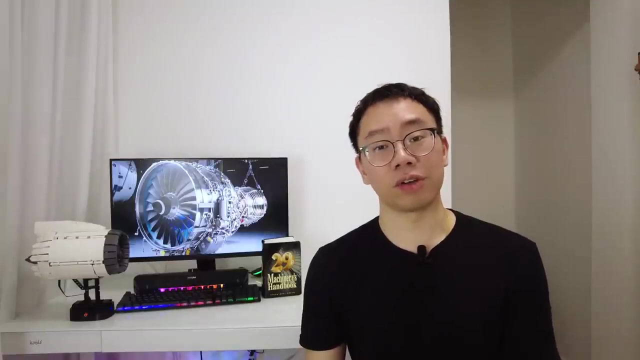 college. it's pretty unlikely. if you have less than one year of industry experience, your salary will likely fall between 70k to 90k depending on your location and company. you'll likely need to have three or more years of experience before hitting six figures the starting salary of software. 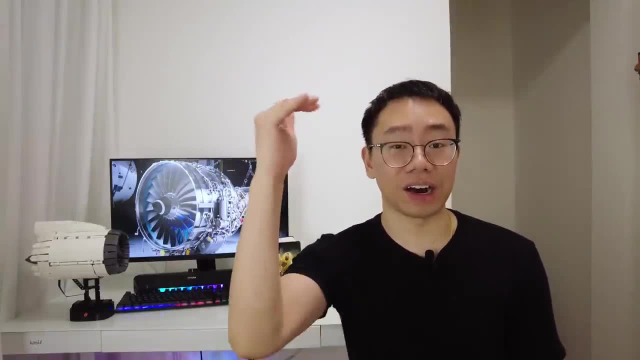 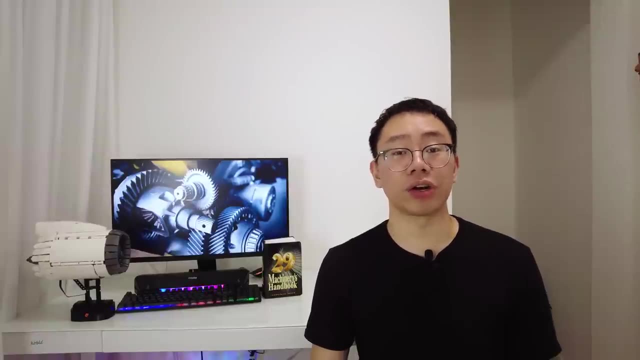 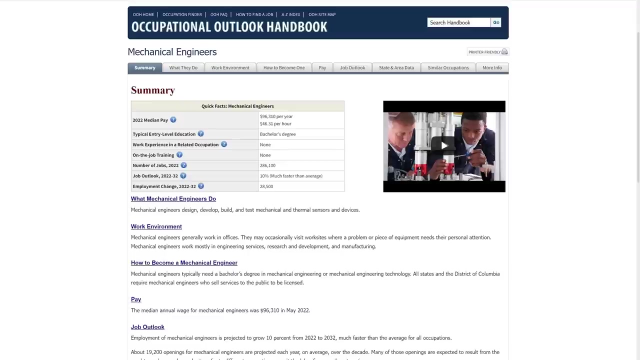 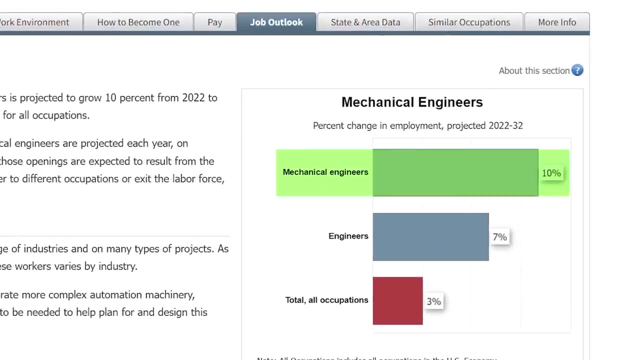 engineers and data scientists will typically be a lot higher. however, if money isn't your top priority, you'll definitely have a lot of opportunities in mechanical engineering for growth, whether you want to stay in a technical track or transition into the managerial track. the number of mechanical engineering jobs in 2022 was 286 100 and it's expected to see a 10 growth rate between 2022.